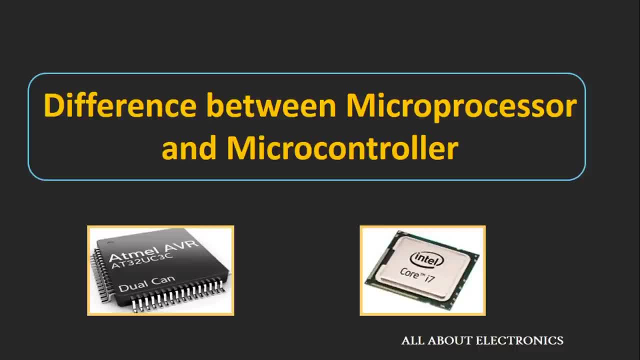 between them. They almost look very identical, But they are different in many aspects. They are different in terms of the applications in which they are used. They are different in terms of the cost. They are different in terms of the processing power which they possess. 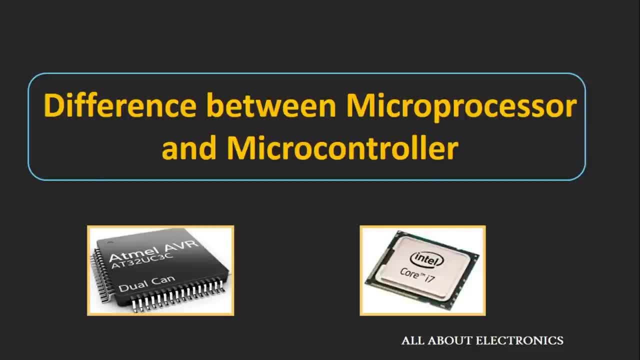 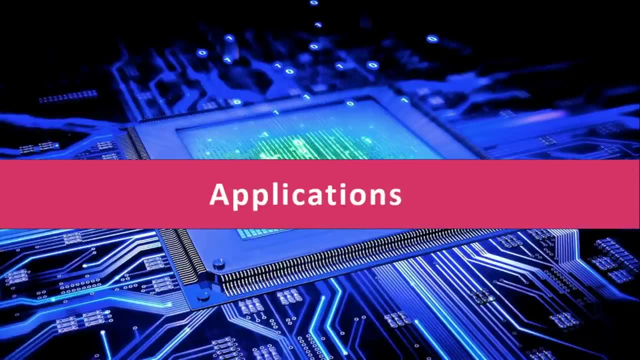 And they are different in terms of the power consumption. So today we will see the difference between the microprocessor and the microcontroller based on all these aspects. So first let's see the difference between them in terms of the applications in which they are used. 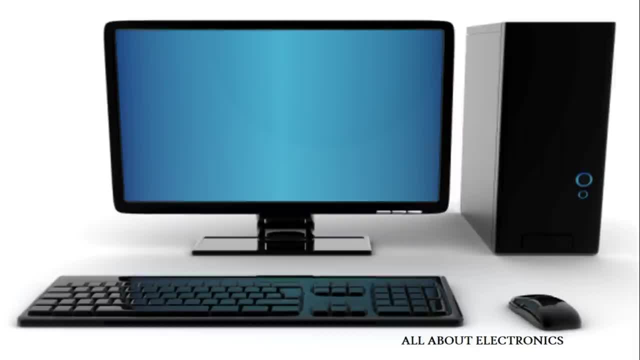 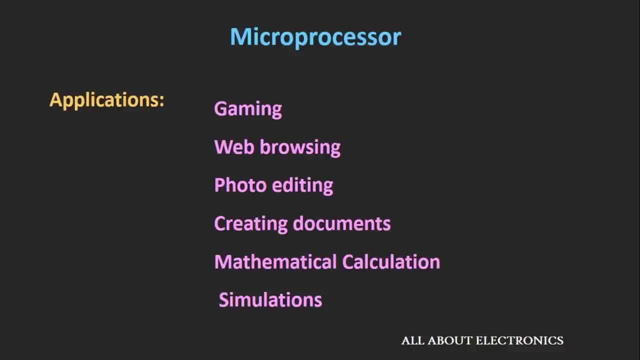 So the classic example of a microprocessor application is a personal computer or a laptop. So using this laptop we can do a lot of stuff Like. we can use it for gaming, for web browsing, for photo editing, for creating documents, Or we can use it for mathematical calculations. 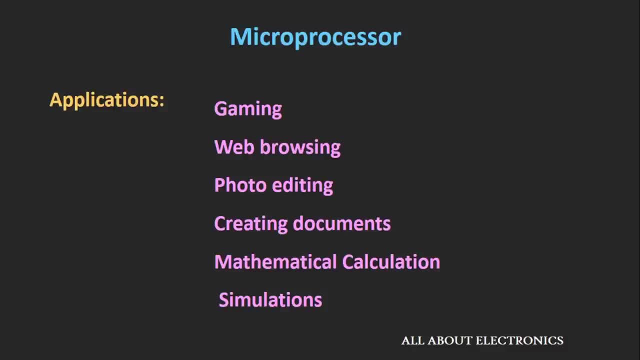 simulations or media streaming. So a microprocessor is basically used in applications where the task is not predefined. It depends upon the user. Or it is used in applications where the task is not predefined, Or it is used in applications where the task is not predefined. 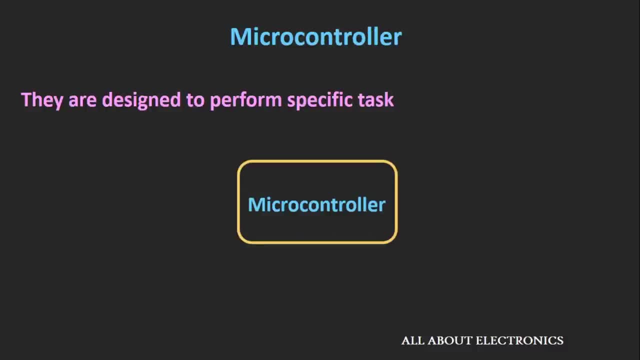 Or it is used in applications where the intensive processing is required, While in case of a microcontroller they are used for a specific task. So, based on the inputs which are given to the microcontroller, it does some processing and it gives the result as an output. So here the inputs could be a user input or 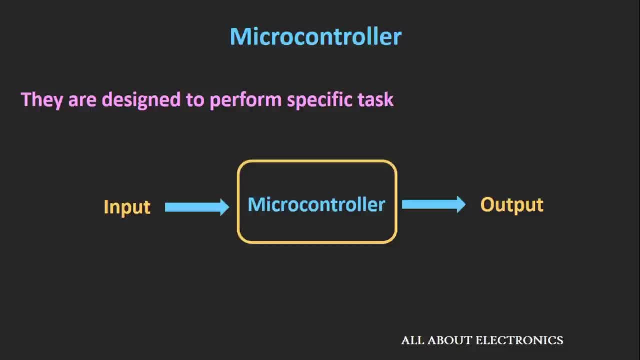 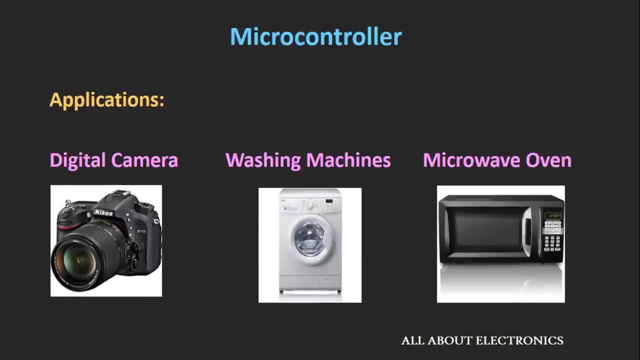 the inputs which are coming from the sensors. So the examples of a microcontroller applications are like digital camera, washing machine and a microwave oven. So if you see all these devices, the task which is going to be performed is predefined, Like in case of a microwave oven, once you set the power and the timing it gives you. 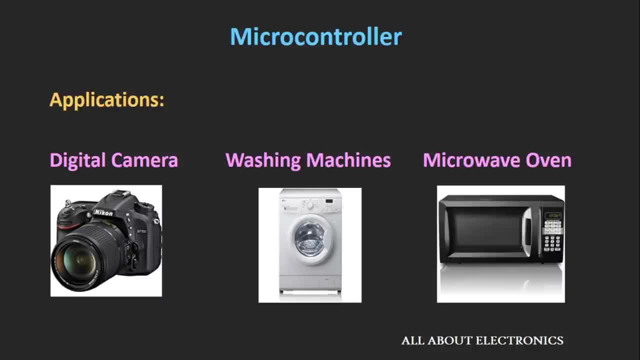 the cooked food. Likewise in the case of a washing machine, once you set the parameters of the machine, it gives you the clean and dry clothes. So, basically, a microcontroller is used in applications where the task is predefined. Now let's see the difference between them in terms of the internal structure. 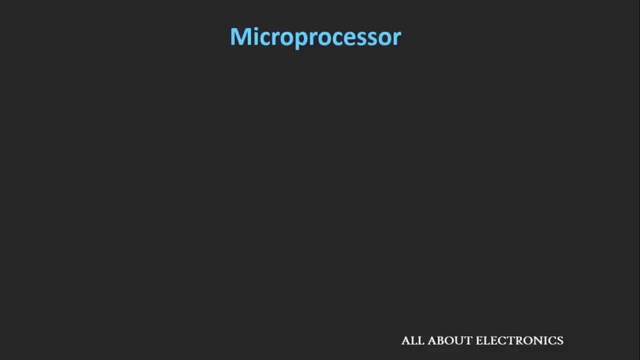 So, like I said earlier, the microprocessors are used in applications where the task is not predefined, So they can be used for a variety of purposes. For example, the microprocessor is used in applications where the task is not predefined. It can be used for a very light application, like creating a document, or very intensive. 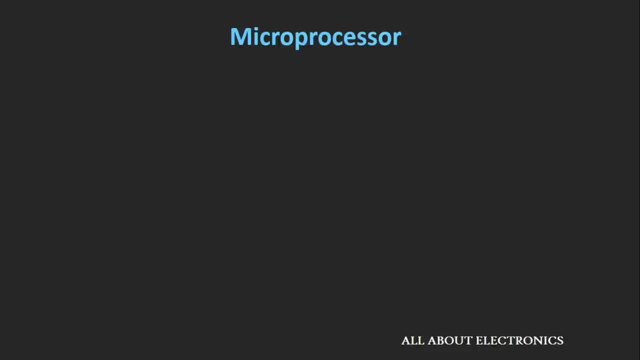 application, like a gaming or a media streaming. So the amount of memory that is required depends upon the application. So if you see a microcontroller chip, it only contains a CPU which is Central Processing Unit, And all the memory elements and the IO interfaces are connected to it externally. 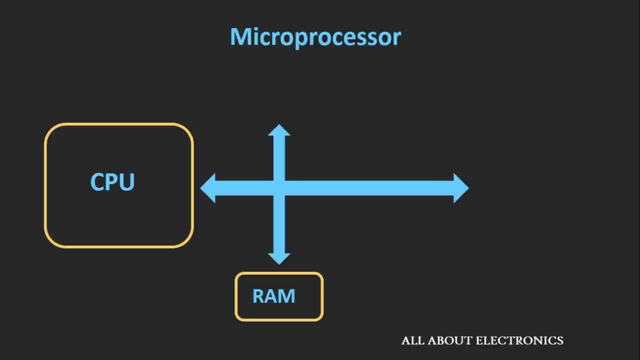 So in case of a microprocessor, the memory elements like RAM, ROM, IO ports, RAM, RAM, RAM serial interface and the timers all are connected externally, While in case of a microcontroller, as they are used for a specific task, the amount of 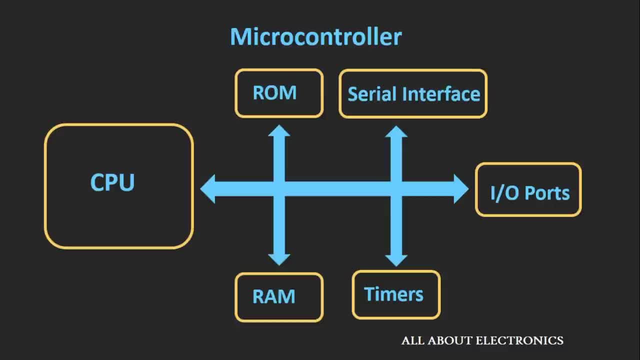 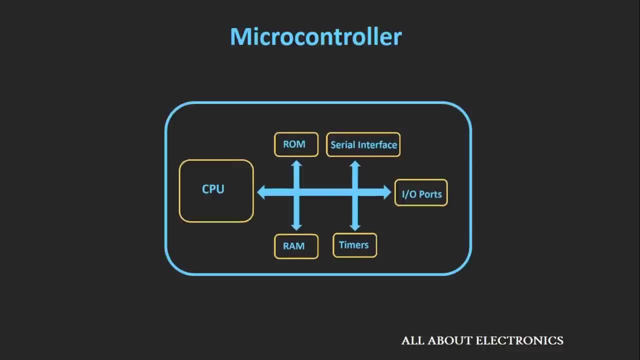 memory and the IO ports which are required are limited, So in the case of a microcontroller, all the memory elements and IO ports are integrated along with the CPU inside a single chip, So the size of the overall system is much. 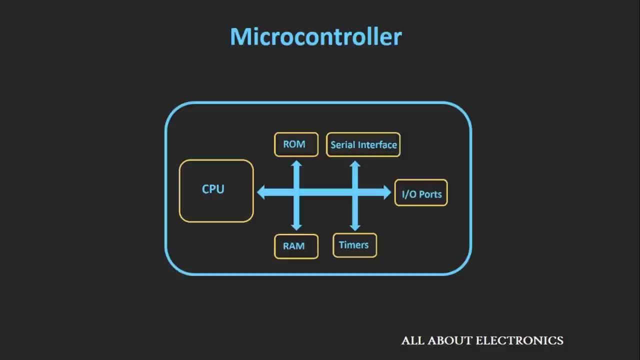 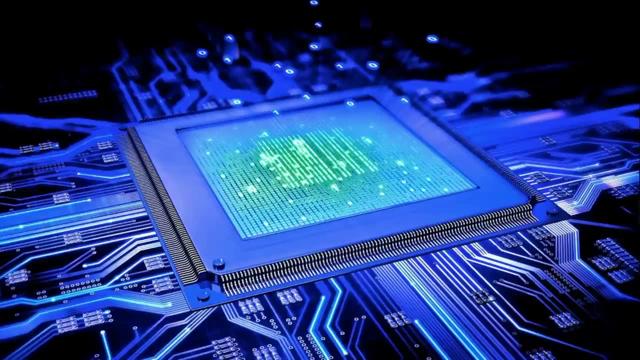 smaller, While in case of a microprocessor, as all the memory elements and IO ports are connected externally, so overall size of the system is much larger than the microcontroller. Now let's see the difference between microcontroller and microprocessor in terms of the processing power and memory. 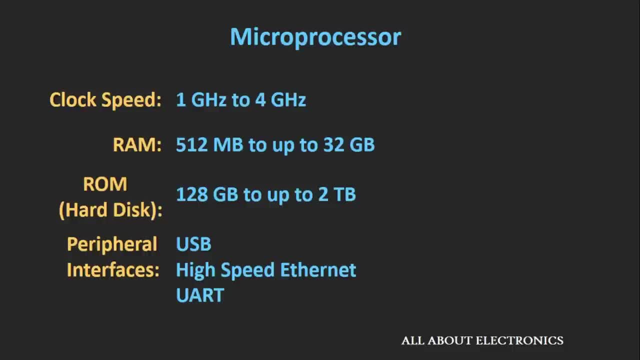 So microprocessors are operated at a much higher speed. So if you see the clock speed of a microprocessor, it is in the range of GHz. The clock speed varies from 1 GHz to 4 GHz for the high-end processors. So as a microprocessor has to run an operating system, the amount of memory that is, RAM. 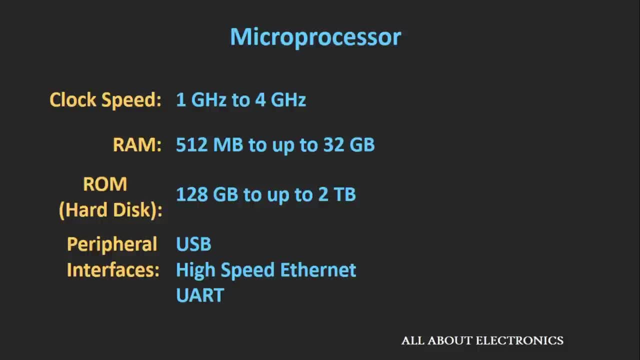 and ROM which is required is quite high. For example, random access memory or RAM, which is a volatile memory, in a microprocessor. it ranges from 512 MB and it goes up to 32 GB in a high-end microprocessor. Similarly, if you see the ROM in the microprocessor, it ranges from 128 GB and it goes up to 2. 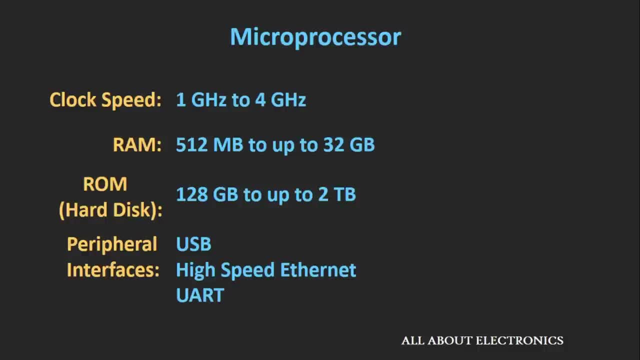 TB, That is 2 TB, And the common peripheral interfaces which you see in the microprocessors are like USB, high-speed Ethernet and the UART, While in the case of a microcontroller it's in the range of GHz. So if you see the clock speed of a microcontroller, 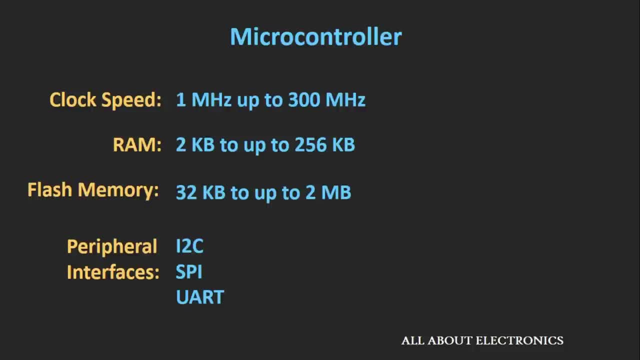 it ranges from 1 MHz and it goes up to 300 MHz in the high-end microcontrollers, And as these microcontrollers are defined for a specific task, the amount of memory that is required by them is quite less. So if you see a random access memory or RAM, 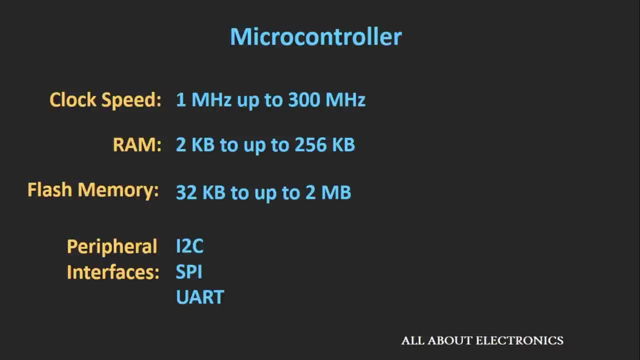 inside the microcontroller it is in the range of KB, So it can go from 2 KB up to 256 KB. Similarly, if you see a flash memory or a program memory inside a microcontroller, it varies from 32 KB and it can go up to 2 MB. 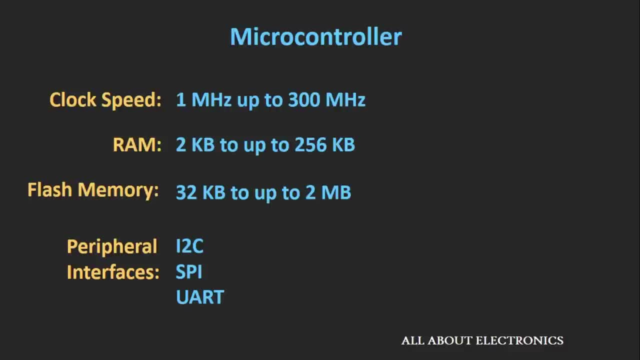 And the common peripheral interfaces which you find inside the microcontroller are like I2C, SPI and the UART. So basically all these are serial interfaces which you find in modern-day microcontrollers. So if you see modern-day microprocessors they are either a 32-bit or a 64-bit. So a 32-bit microprocessor means a microprocessor. 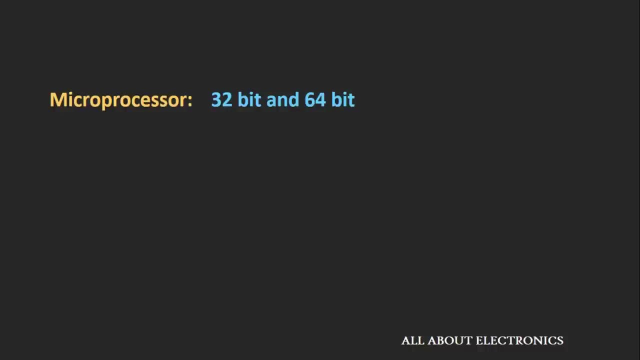 can handle a 32-bit microcontroller And if you see a 32-bit microprocessor, it's a 64-bit microprocessor. So in a 64-bit microcontroller it can handle a 64 bits of data at the same time. Similarly, a 64-bit microprocessor can handle 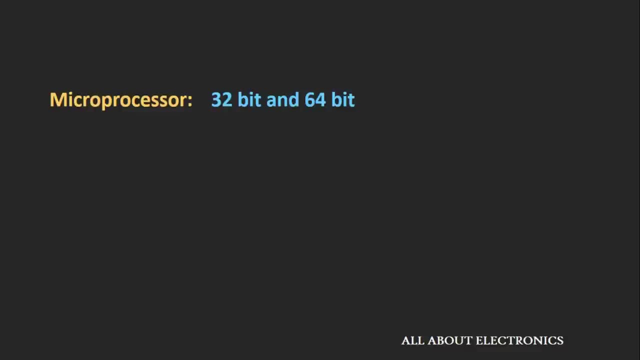 a 64 bits of data at the same time. So, in case of a 64-bit microprocessor, all the address bus and the database are of a 64 bits. Similarly, in the case of a 32-bit microprocessor, the address and the data bus are of a 32 bits. 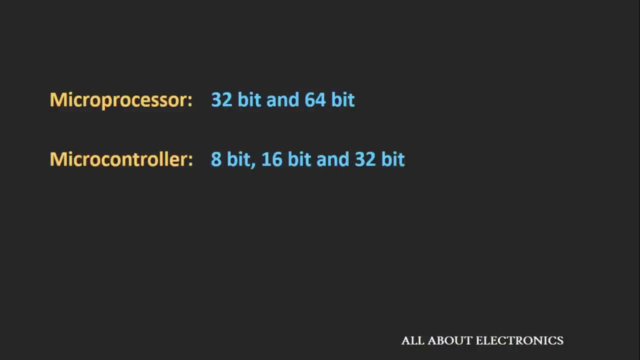 While if you see a modern-day microcontrollers, they are either of 8-bit, 16-bit or a 32-bit. So the amount of data which can be handled by a microprocessor in a single cycle is higher than the microcontrollers. 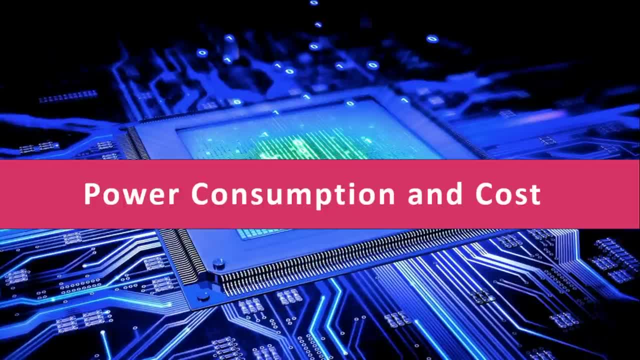 Now let's see the difference between the microcontroller and microprocessor in terms of the power consumption and the cost. So in case of a microprocessor, as all the memory elements and the I-O ports are connected externally, the overall cost of the system, as well as the power consumption, is higher. 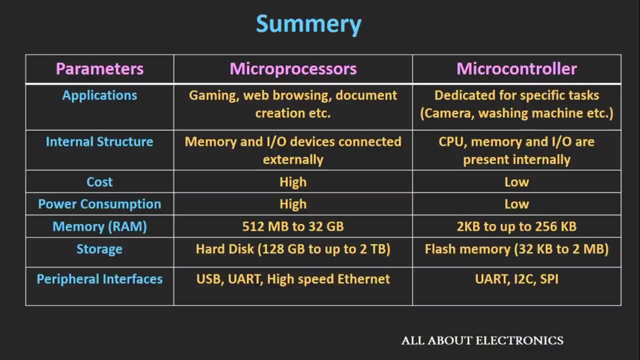 compared to the microcontrollers. So this is a summary of the differences between the microprocessor and the microcontroller, based on the various parameters which we have already discussed. The downloadable link for the same is given in the description below, So you may check that out. 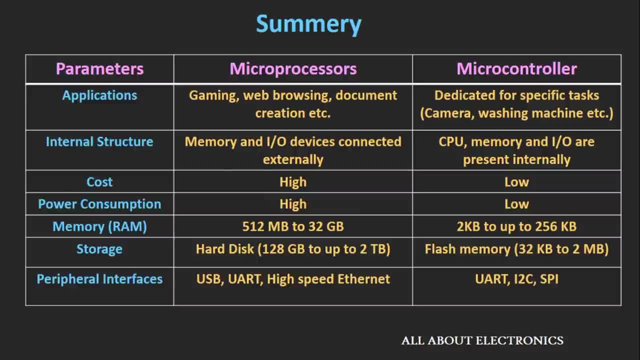 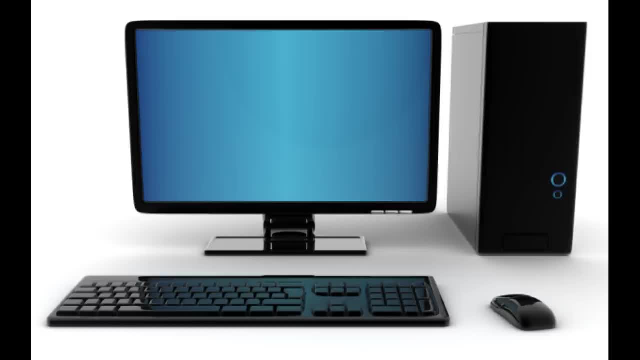 So, before I end up this video, one more thing which I want to tell you is that you might have observed that when I was discussing about the applications of the microprocessor, I had given the example of a personal computer, But I didn't mention anything about the smartphone.